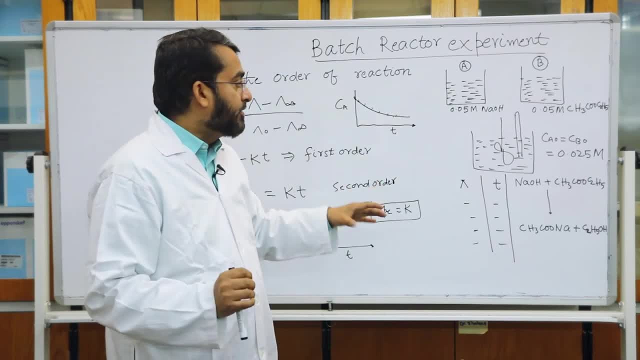 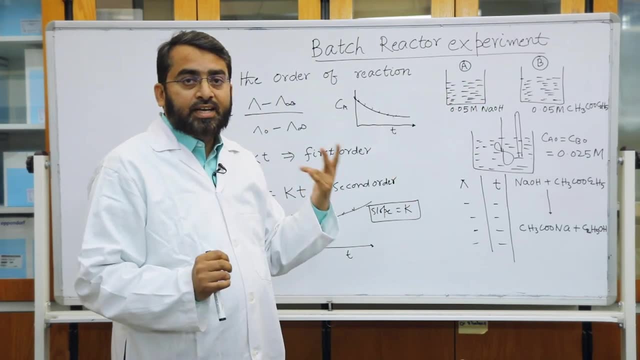 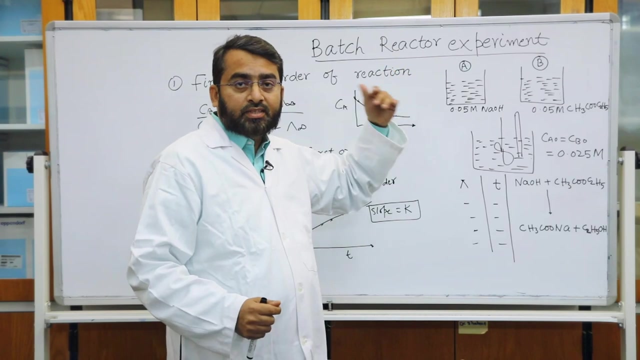 for 5 minutes, suppose. Then again we repeat it and we heat the reactant- both of them- and we conduct at high temperature and we get the conductivity graph for other temperatures, So like this is at 20,, 25,, 30,, 35 and so on. 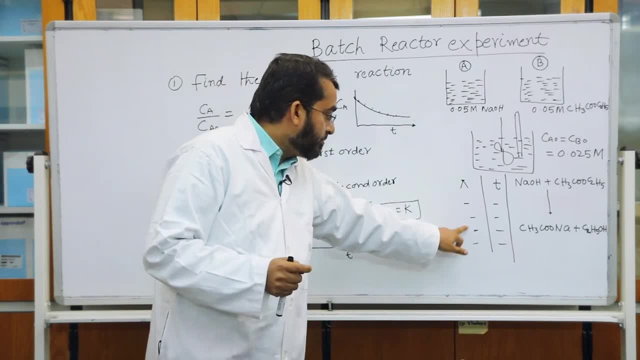 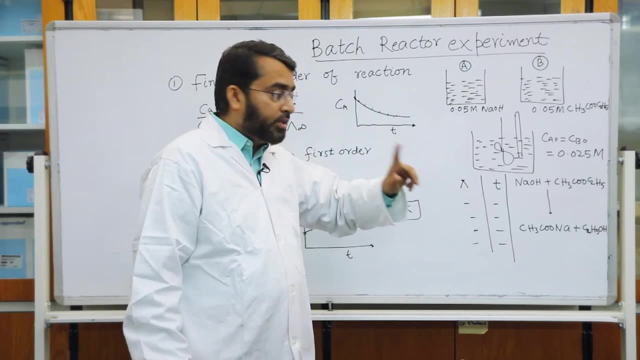 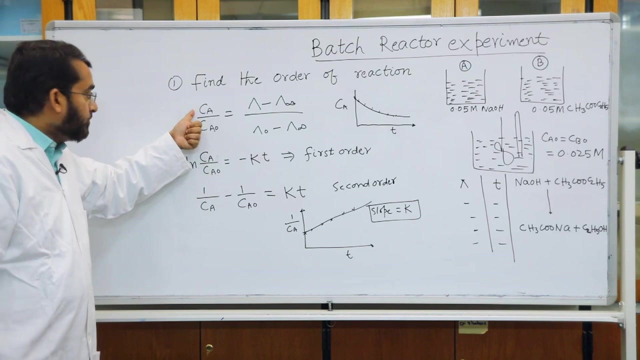 So once you have the data- conductivity versus time- you have to process it. So I will just explain to you how to process this data. You know that how to convert conductivity to concentration, Using this equation, you can convert connectivity to equation. This is a measured connectivity. 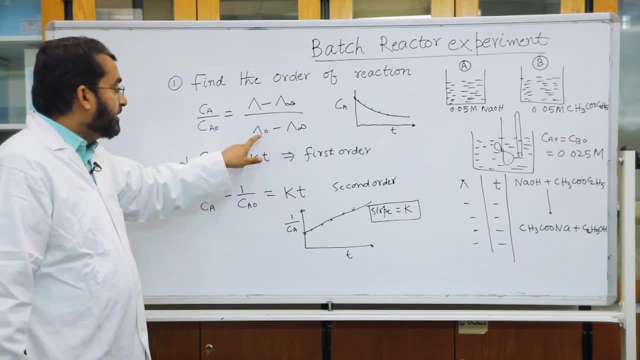 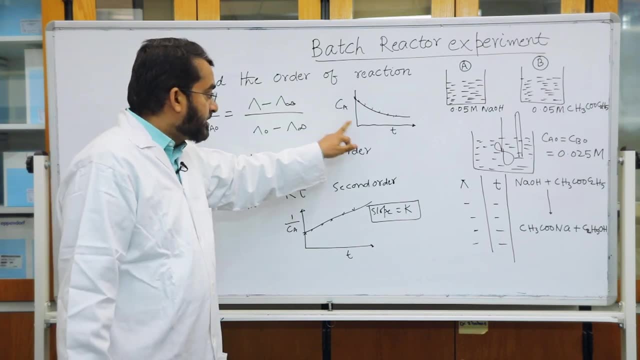 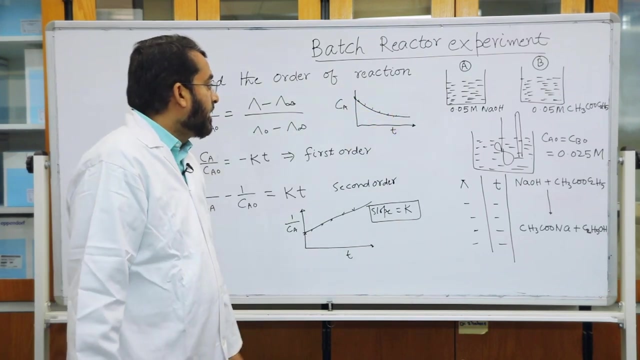 with time. lambda 0 and lambda infinity are initial and final connectivity. So once you know the concentration, you can plot concentration versus time graph and you can see A is a reactant, so it is decreasing with time and makes sense And you can see that the slope is initially. 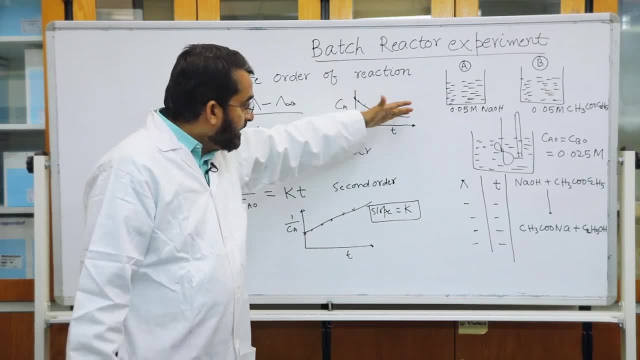 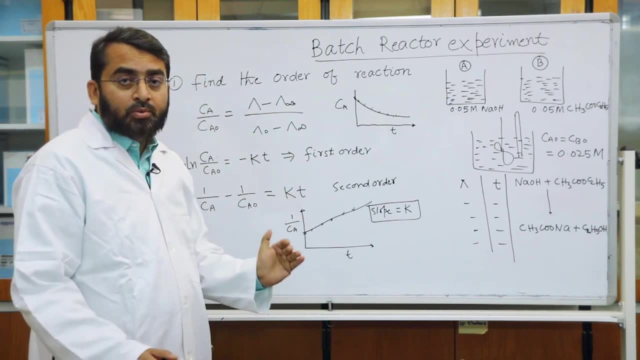 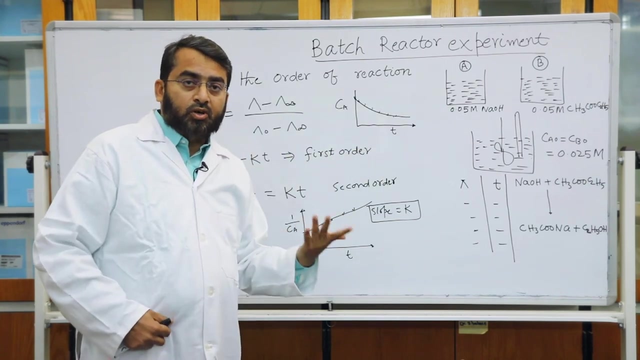 it is higher because rate of reaction is higher and slowly rate of reaction almost is zero because all the reactants are being consumed. So now your job is to find the order of the reaction. So CAT graph is there. you look for different type of order, what equations you have. So if you search you will find. 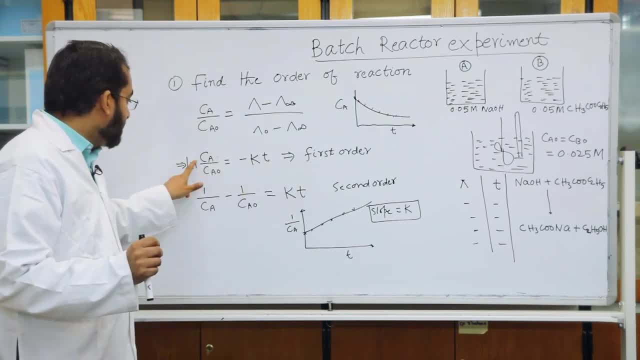 this is the equation for first order: ln. CA by CNR is minus KT. Try to fit this curve and you will find that this is the equation for first order. ln. CA by CNR is minus KT. Try to fit this curve and you will find. this is the equation for first order: ln. CA by CNR. 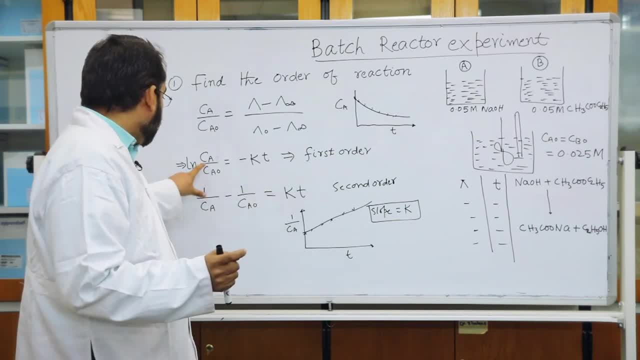 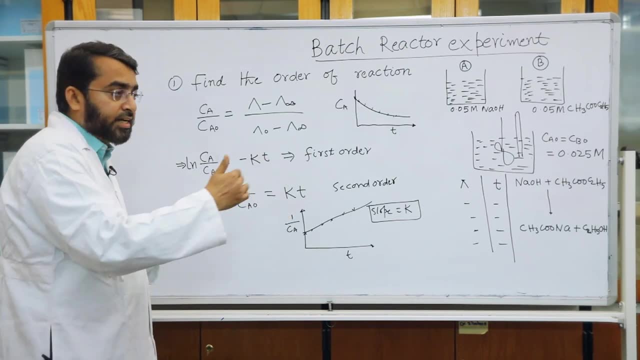 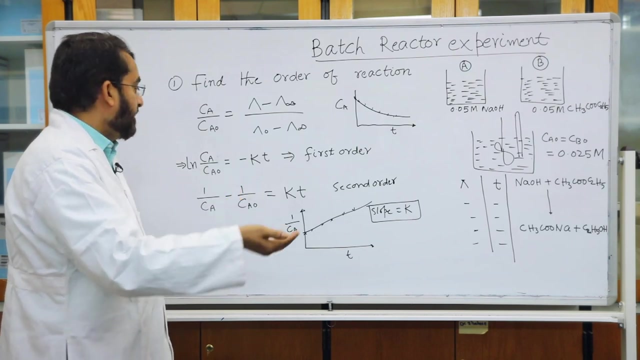 is plus KT. Try to connect them in reverse. You can see whether it is linear or not. Plot this, this versus time. If it is linear, then you can say: and look at the value of R square in Excel. you can say that this is first order or not. Come to the second equation, which? 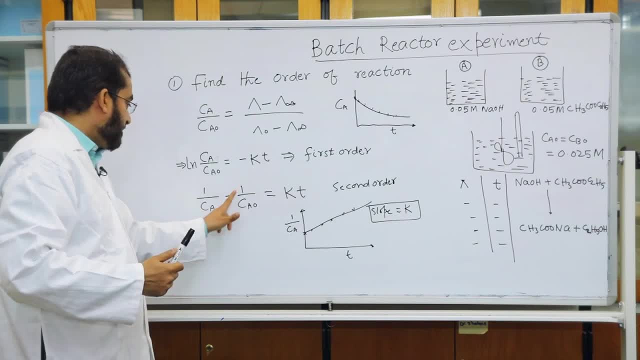 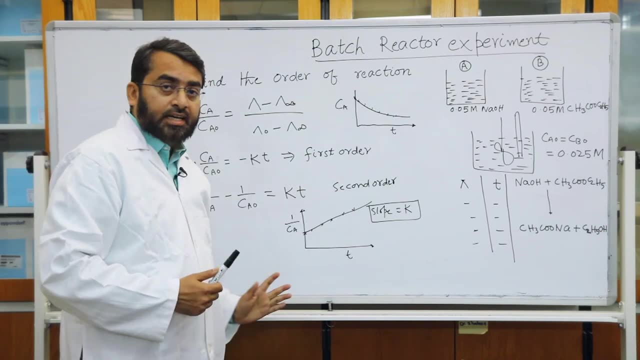 is this second order equation: 1 over CA minus 1 over CA0 equals KT. So you get something like this. It is linear, R square is close to 1, you can say that our equation is second order. okay, And slope. 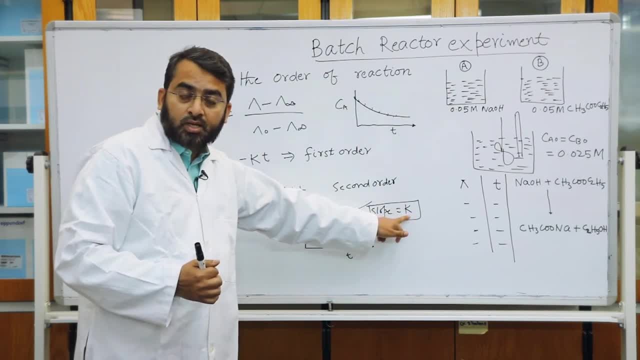 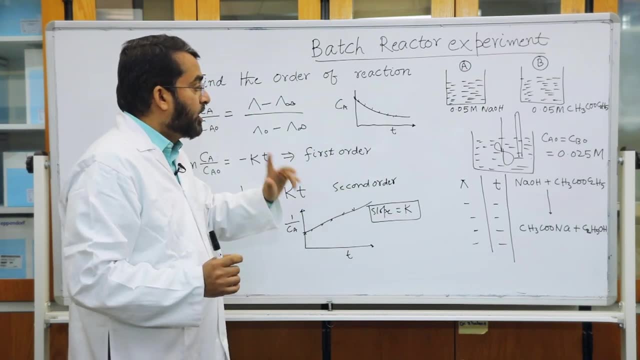 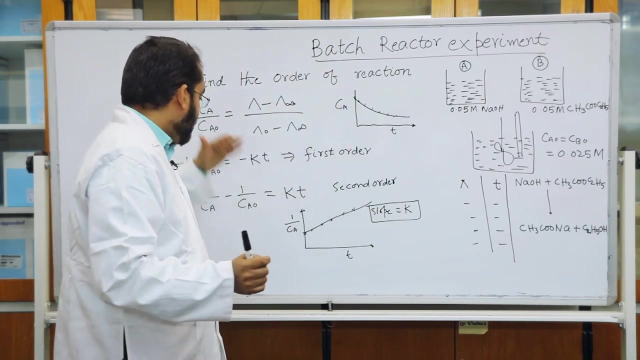 of the curve will give you the rate constant value And in this way you can calculate the rate constant value at different temperature. you repeat same thing. you have the data for all. you have connectivity versus time data for other temperatures. repeat the same thing. 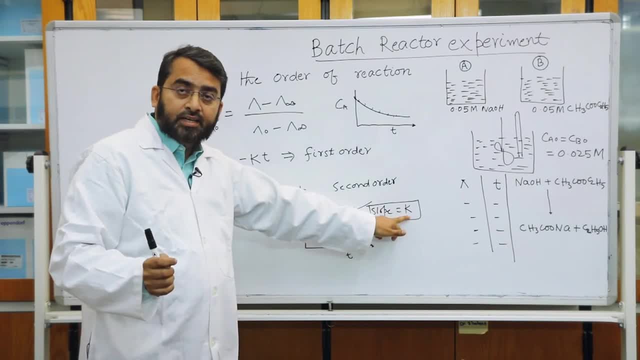 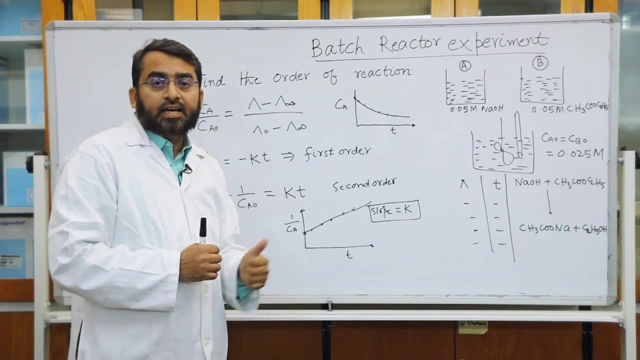 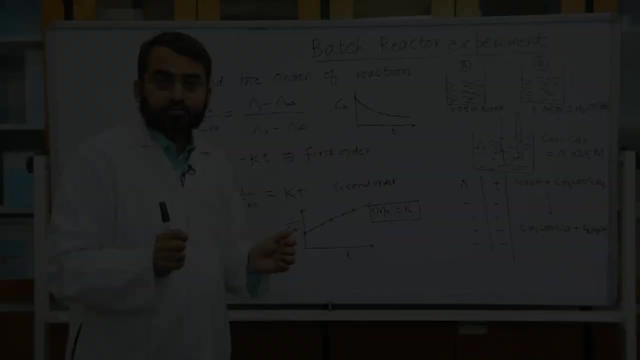 repeat the graph, get the slope value k, and you will get k values at different temperature, and then, using Arrhenius equation, you can find the activation energy for the reaction. okay, That is it. I hope it is clear. thank you. We are going to conduct experiment batch reactor, as I explained to you, So we have reaction. 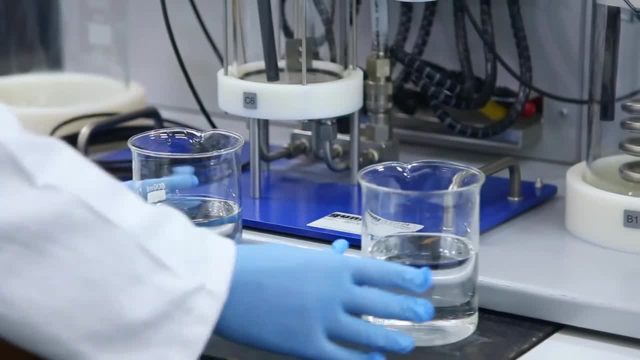 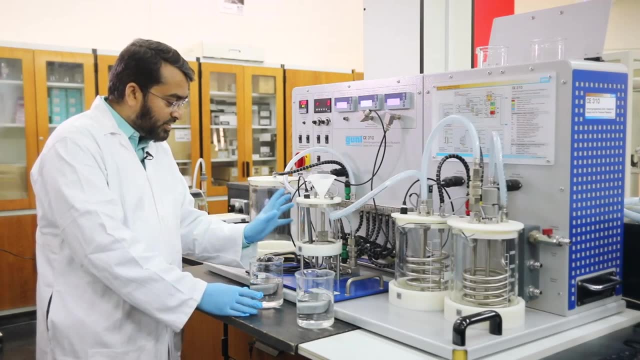 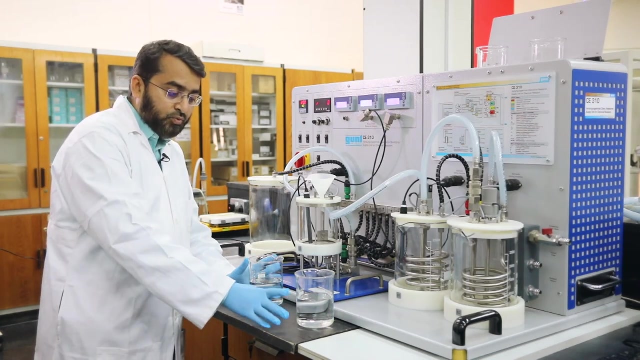 between sodium hydroxide and ethyl acetate. okay, So I am going to mix this in the reactor now, And this is your batch reactor. this capacity of batch reactor is less than 1 liter. So what we are going to do? we are going to mix 400 milliliter of sodium hydroxide and 400 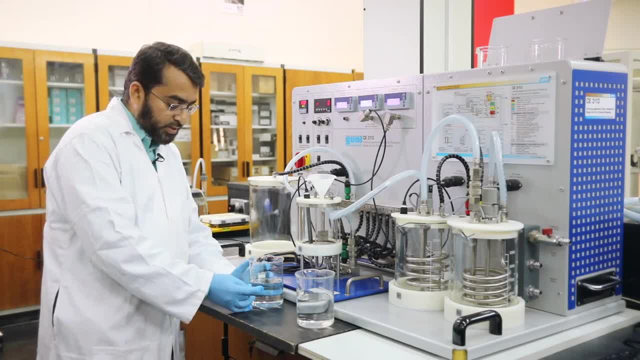 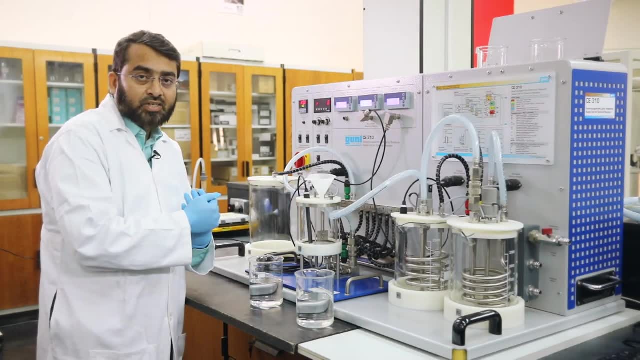 milliliter of ethyl acetate. The concentration here is 0.05, 0.05.. When we mix it, volume will be doubled, so your initial concentration will be half of the 0.05.. So you will be starting. 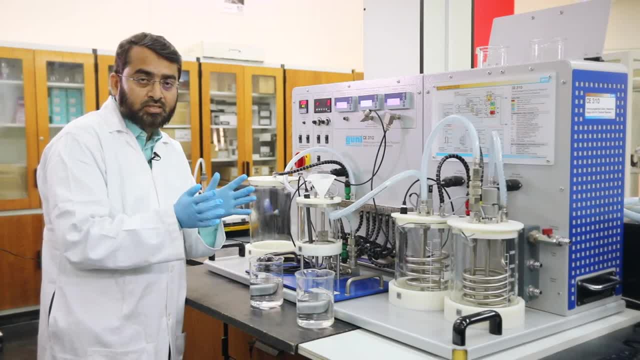 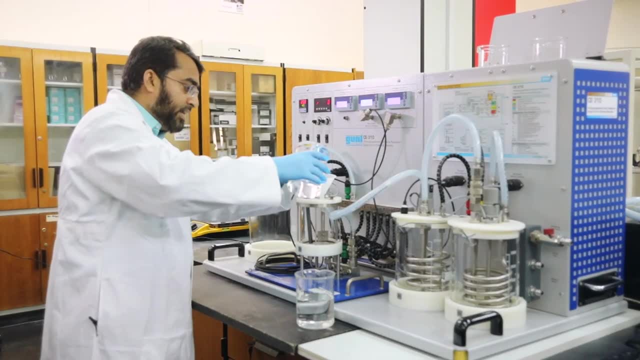 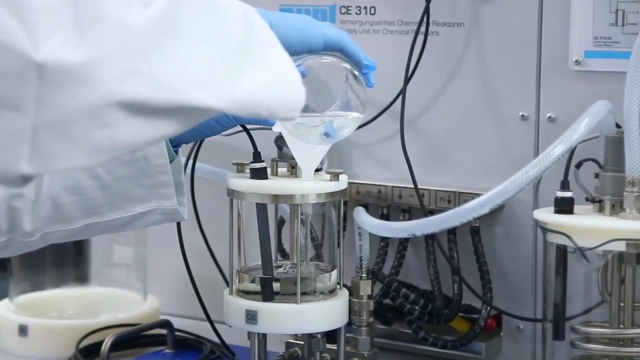 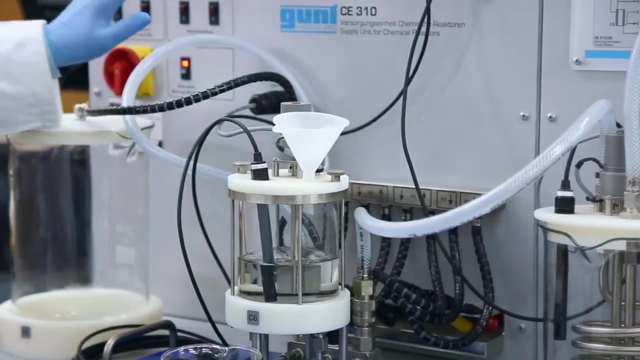 with the concentration: Ca 0, Cb 0.. 0.025 molar. okay, So this is sodium hydroxide. I will add this first in the reactor. okay, Let me start the stirrer. and now you can see the conductivity values is rising. yeah, because 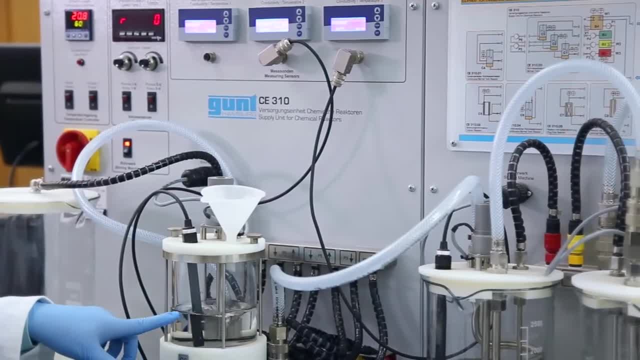 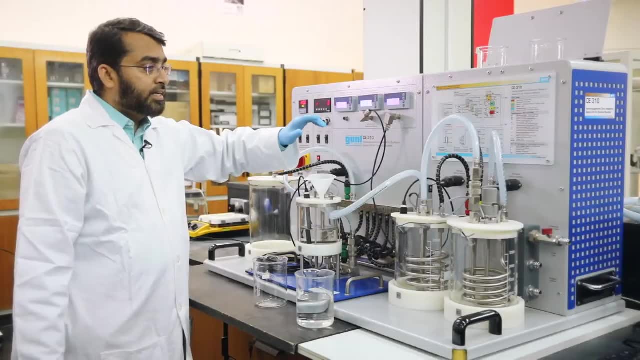 this sodium hydroxide is conductive, So it has been connected to the reactor, So it has conductivity and it will go. it will become constant. now with this concentration, We are conducting this experiment at room temperature, So you can see the temperature is around 21,. 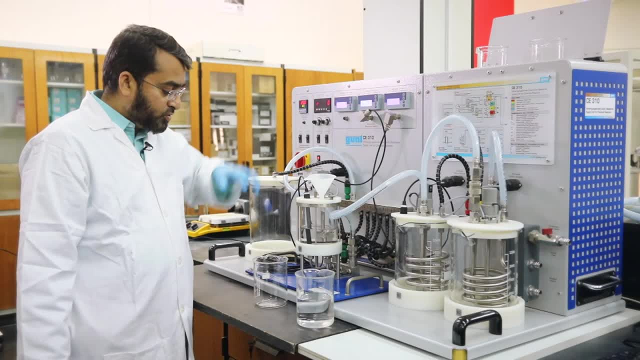 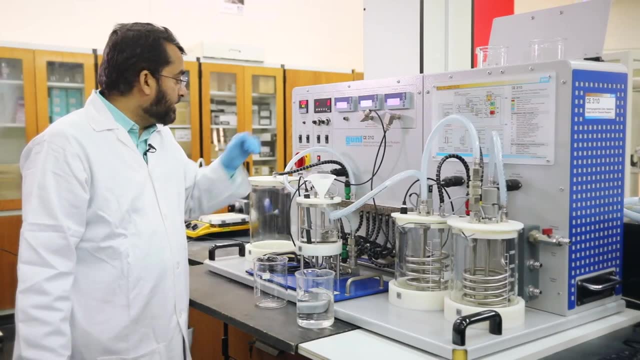 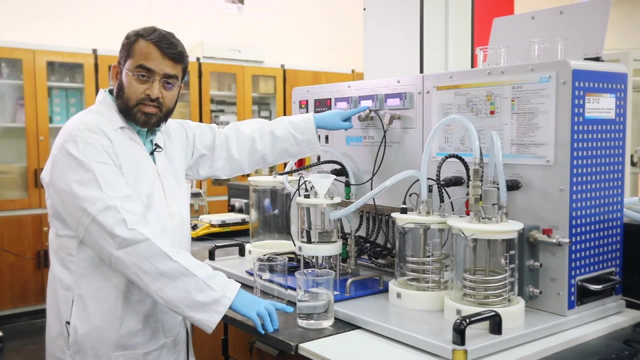 okay, So this is stable. now, This is the conductivity of 0.05 molar NaOH. okay, Now, once we add this one, ethyl acetate, the volume will be doubled. So this is the concentration of sodium hydroxide. okay, And the conductivity will be half, because ethyl acetate doesn't have 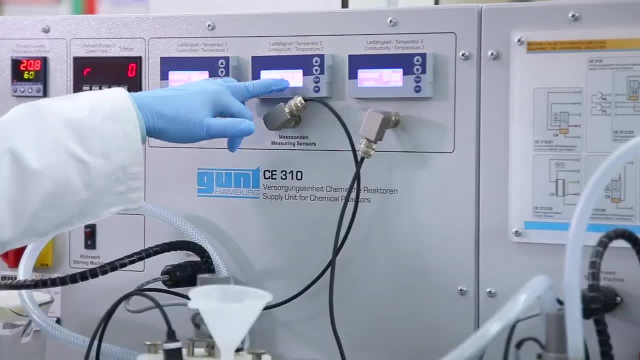 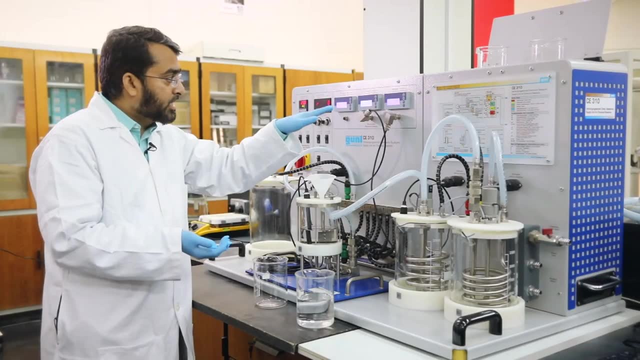 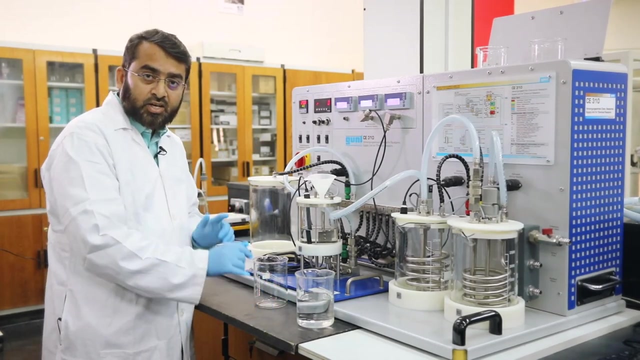 conductivity. So once we mix it the conductivity becomes half. It means mixing is complete. From there reaction starts. So again you will see that connectivity is decreasing because of reaction. So reaction between sodium hydroxide and ethyl acetate started. Sodium hydroxide. 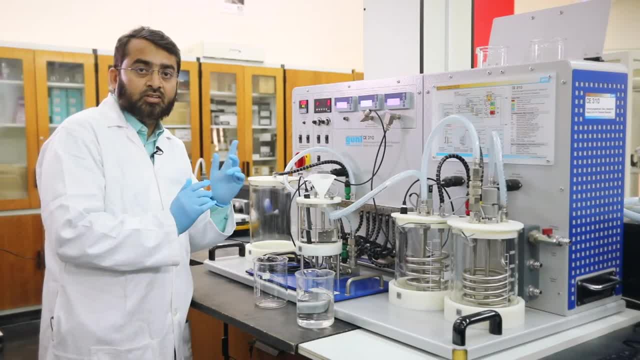 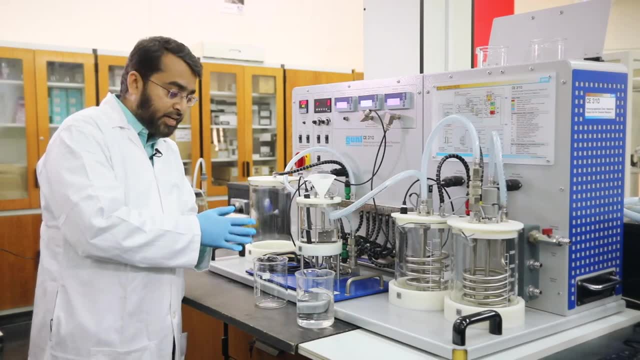 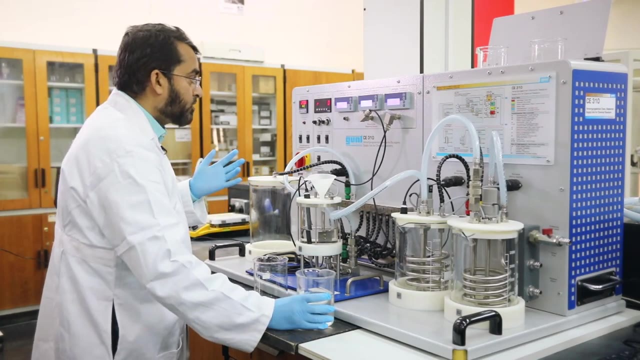 is being consumed. You are getting sodium acetate, which is also conductive, But what? the conductivity of sodium acetate is much less than sodium hydroxide. So with reaction you will see that conductivity will decrease with time. okay, So I will add this ethyl. 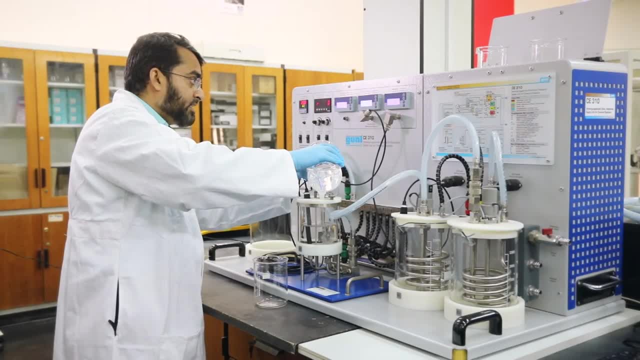 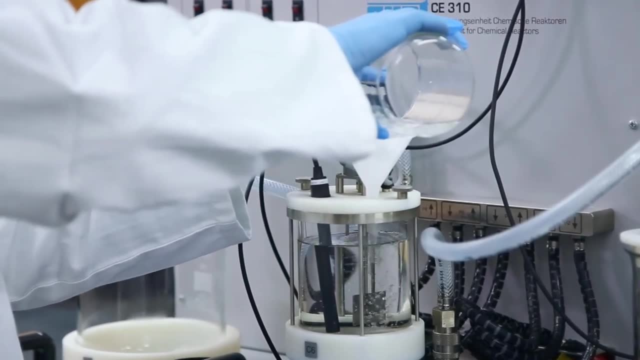 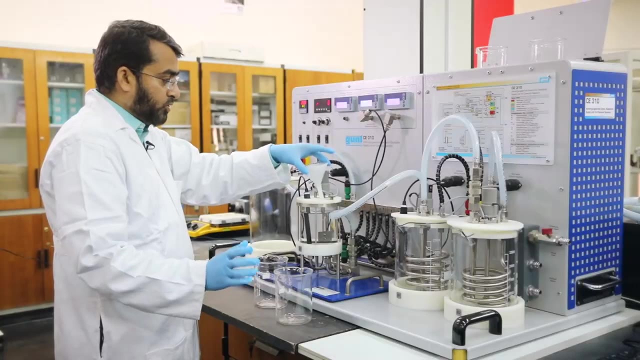 acetate. now You can see the conductivity start decreasing because it is diluting sodium hydroxide And after mixing it will be almost half of the previous value. So we started around. it will be 5.. So you can see the data already is being taken there in the software. 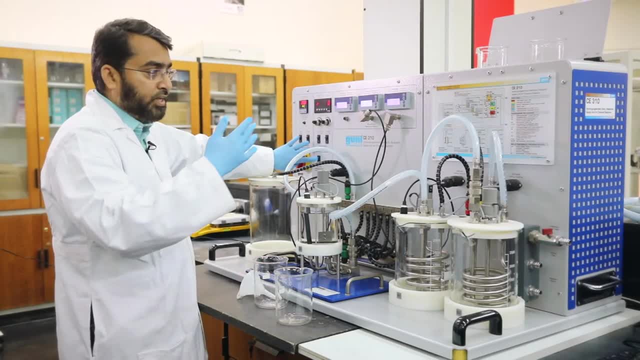 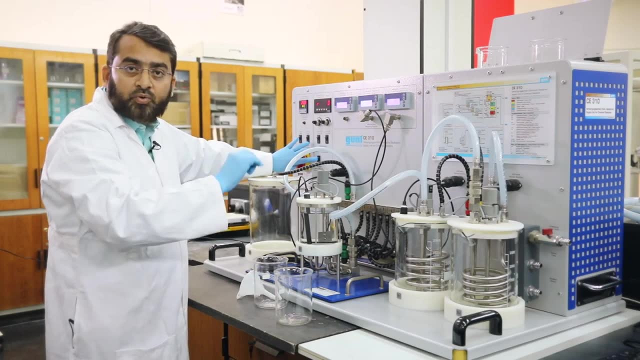 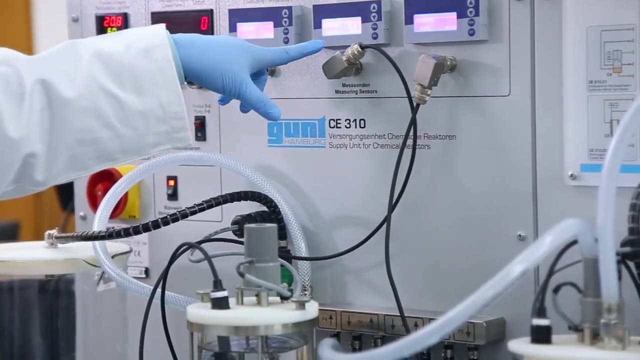 And then we start the stirrer. After the half value of conductivity of previous value, you can say that this is the time- t equals 0- where reaction started. okay, So now we can see almost half of the previous value. Reaction started. Conductivity is decreasing. 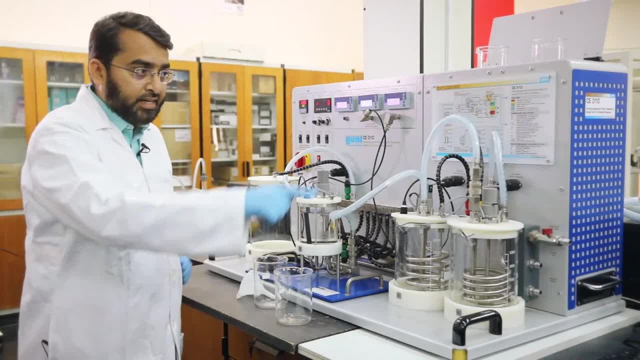 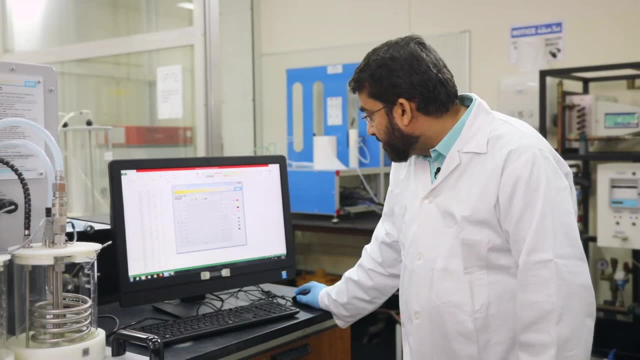 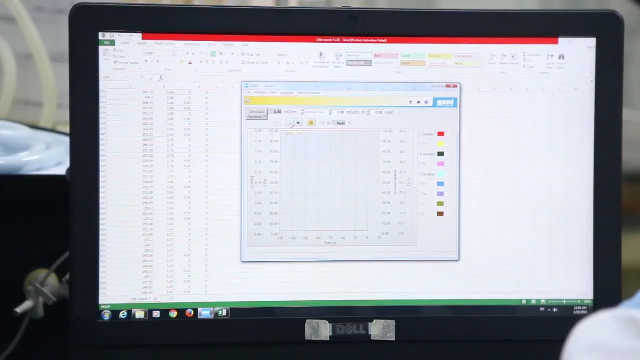 with time, I can show you the in graph. You can see that the software is taking the data of the conductivity- What is this time? And we can export this data to Excel. export data to Excel, okay, and give the file name and so on. 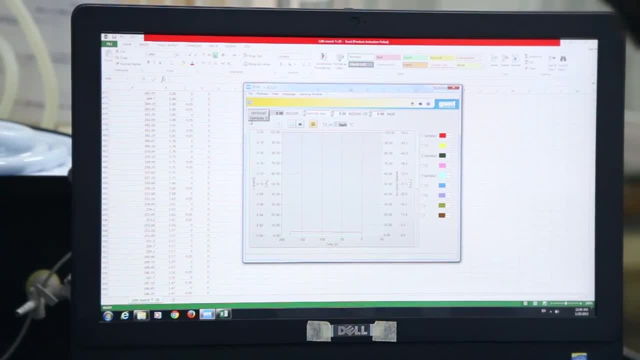 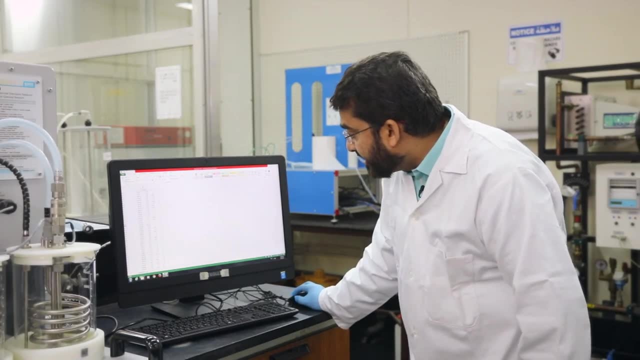 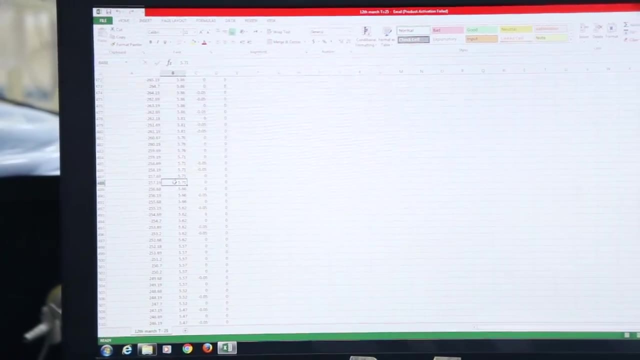 So you can see, you will have data like this in Excel And you can see the initial conductivity is high and here we can say that almost is half of the previous value, connectivity value, as I said, and then you can assume that time t equal to 0 where reaction is started. 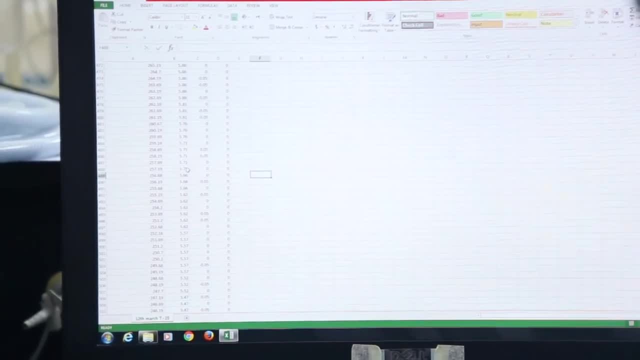 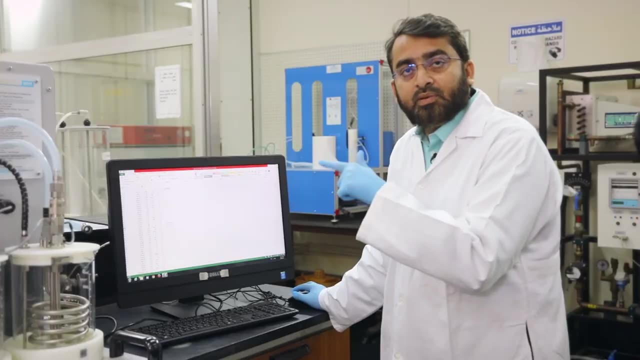 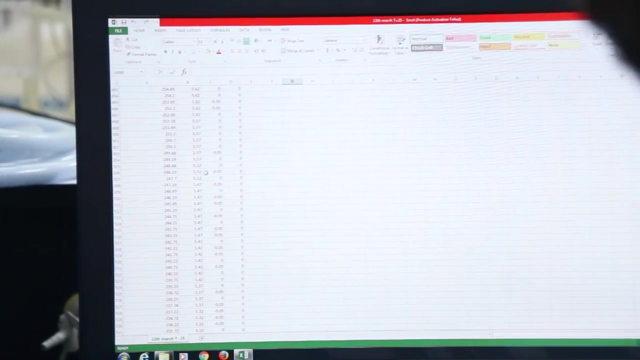 So, from here, take this value and assume is lambda 0, and then convert this data to concentration using value of lambda 0 and lambda infinity, which is constant at the given temperature, and then process this data versus time, and so you will get the concentration versus time.